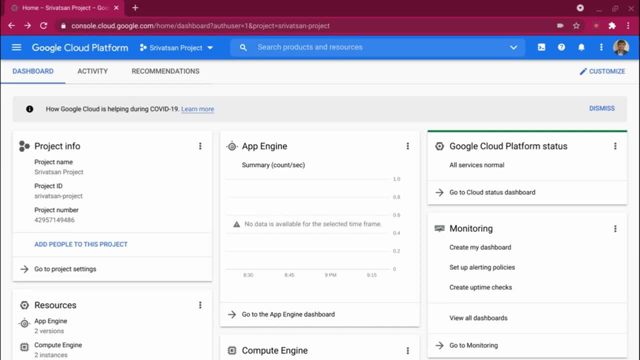 Web Services as well as Azure. Very recently, they launched the service on Google Cloud Platform itself, and what we are going to see is how we can quickly get started with Databricks on Google Cloud Platform Now. Databricks as such is a cloud-based data engineering tool used for processing and transforming massive 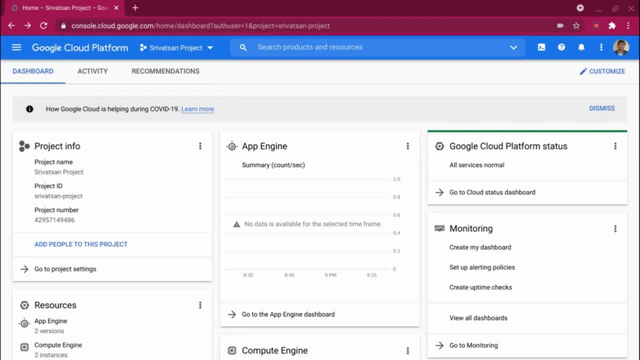 quantities of data and also exploring the data through machine learning models. It also provides a managed Apache Spark environment and Google, by default, has Google Dataproc, which provides a managed Apache Spark environment as well as you can run Apache Spark on an VM or even on an. 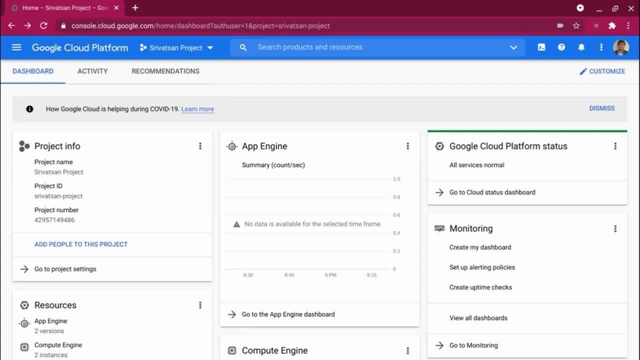 Kubernetes platform. But Databricks is one other option that provides a managed Apache Spark and it also provides an hybrid environment. so if you today you are running on AWS, tomorrow you want to go on GCP, you can just lift and shift your Apache Spark job running on Databricks on AWS or Azure, to GCP or 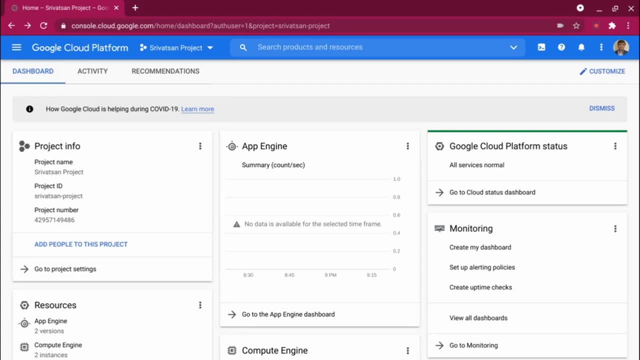 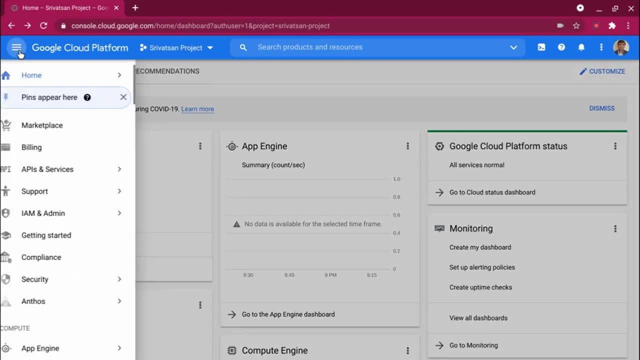 vice versa. So let's get started and see, like, how we can do that. So when you go into Google Cloud Platform, you click on. it is a main dashboard. you click on the menu on the left hand side and scroll down to partner products. if you scroll completely down, you will see like partner solutions and you will see. 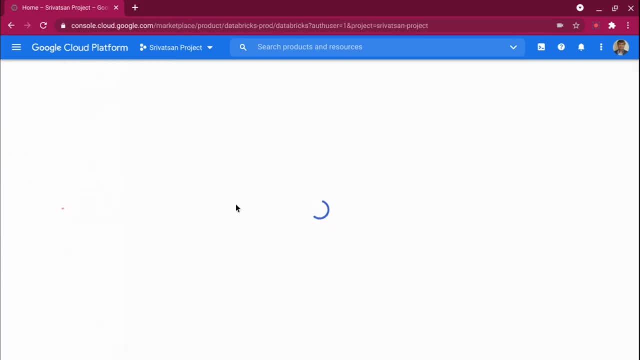 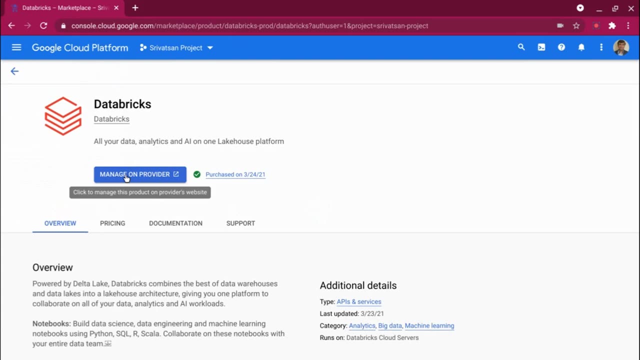 Databricks over there. so click on Databricks now. if this is the first time you are using Databricks, you will see like a purchase option here. I have already done the purchase option, so I'm not seeing it. so you'll see the purchase. 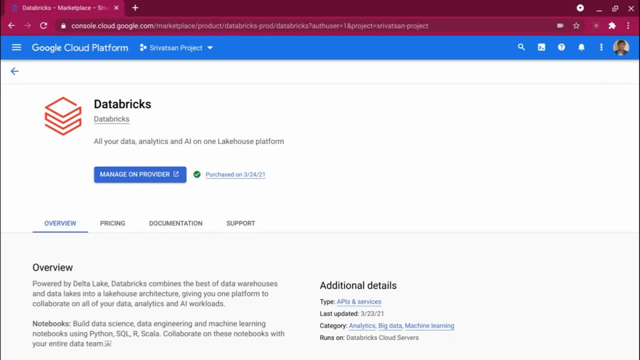 option here for one month. it is free now because they are in a preview mode so you can go and use it and see it, but otherwise you will see a purchase option for me. once I have clicked on purchase, you will see a manage on provider option. so what I am going to do is I'm going to click manage on provider and it will. 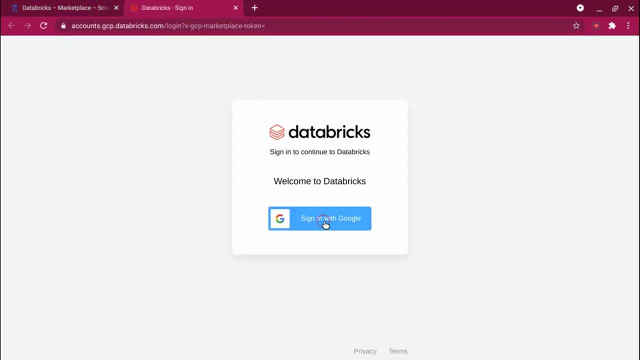 basically take me to the Databricks workspace. so let me sign in with Google, the same ID that I am using to log into google cloud platform. so once you go, it will take you to the authorization page, It will take you to the Databricks workspace and then you can see the workspace details over here now. 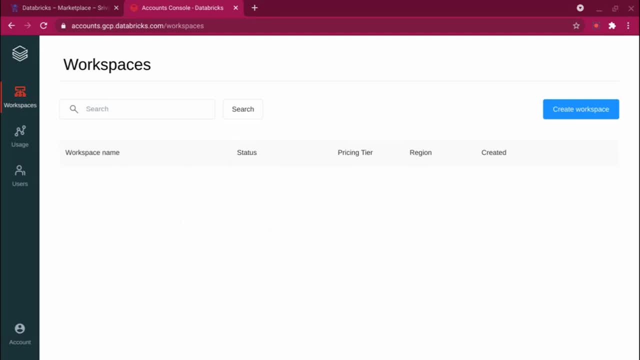 workspace is nothing, but it's an environment for accessing all your Databricks asset. the workspace basically organizes your notebooks, libraries and experiment into folder and it also provides access to data and computational resources. that has cluster and jobs, so you will see like how we can do that. so 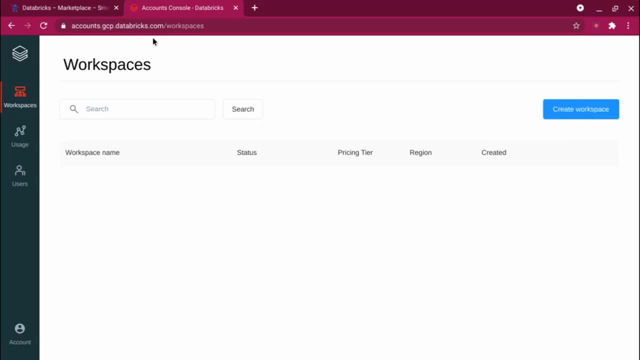 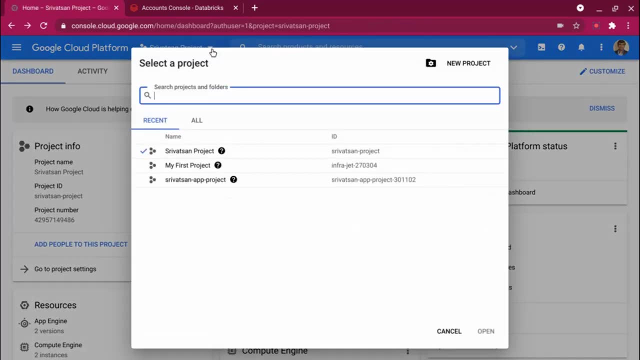 the very first thing is we have to create a workspace over here now. before creating a workspace, let me go back to the Google Cloud platform and let me create a new project. you can use any of the existing project. I'm going to create a new project. the reason for creating a new project is basically show you what 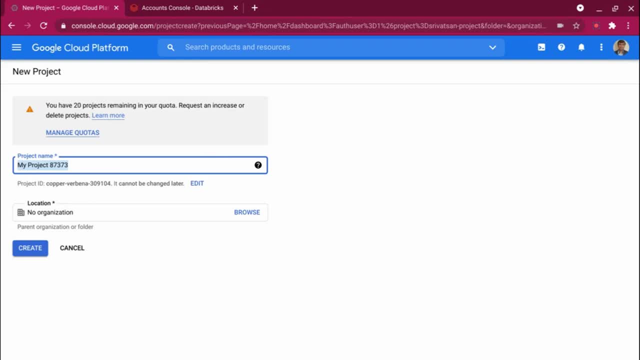 are the access required for the Databricks environment to work. so let me just make it as a Databricks hyphen project, let me give it a name and let me create a new project. so now the product, now that the project is created, what I'm 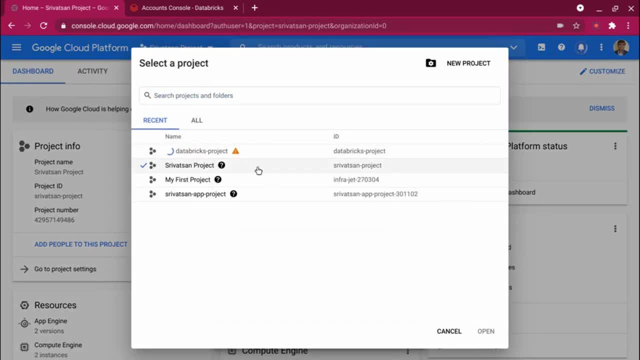 going to do is I'm going to create a new project, and I'm going to create a new project and I'm going to switch to the Databricks project. the project is getting created still, so let me wait for it to get completed and let me have what. 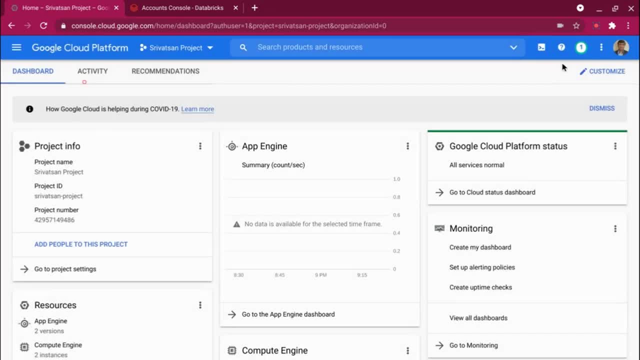 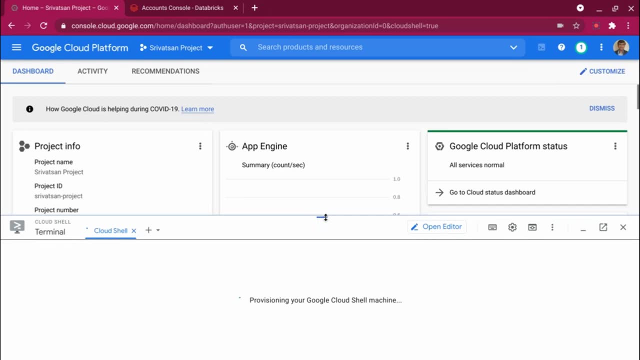 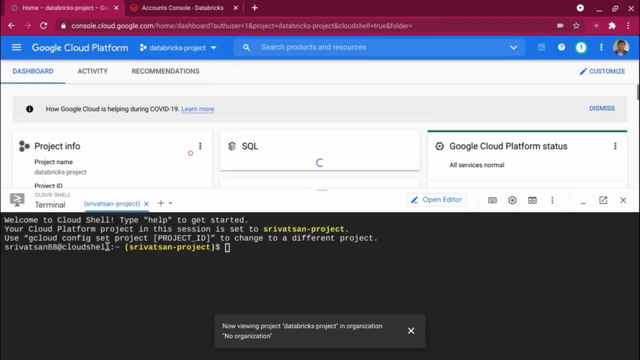 I will do is I'll switch to that particular project, okay, and I will also open my Google Cloud console over here to give all the permissions to the project. that's why I'm also using Google Cloud console, or Google Cloud shell, rather, and let me now select the Databricks project and let me go and 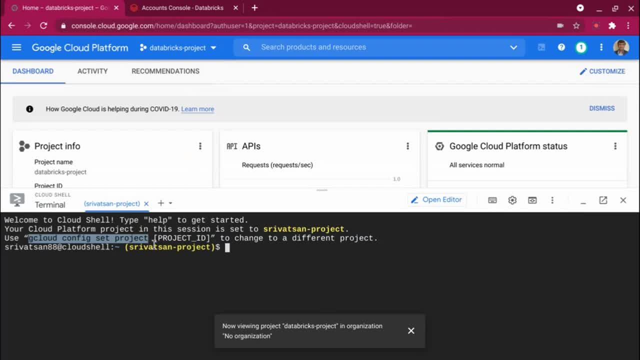 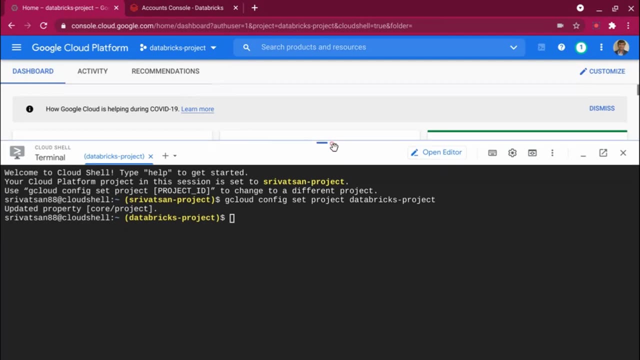 change the cloud shell project over here to the Databricks project. so let me do a ctrl-c, ctrl-b and select Databricks hyphen project. so now, basically, the shell is set to the database project. I'm going to give couple of access to this project. now. what happens like when you spin? 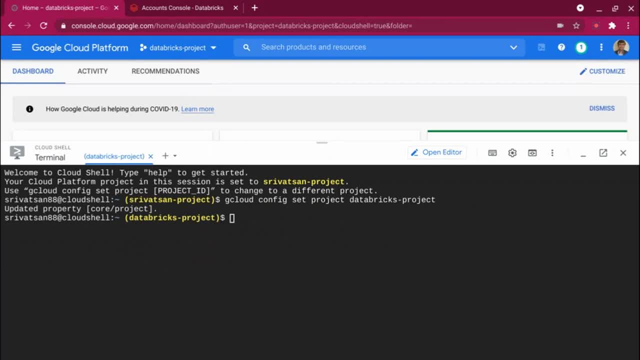 up and up a cluster in Databricks in the back-end. it's going to use Google Kubernetes engine and for that to work, this particular project needs access to compute engine and container engine and I'm going to run a setup aspire engine and container engine and I'm going to run a setupandebee enterprise project is going to use Google Kubernetes engine and for that 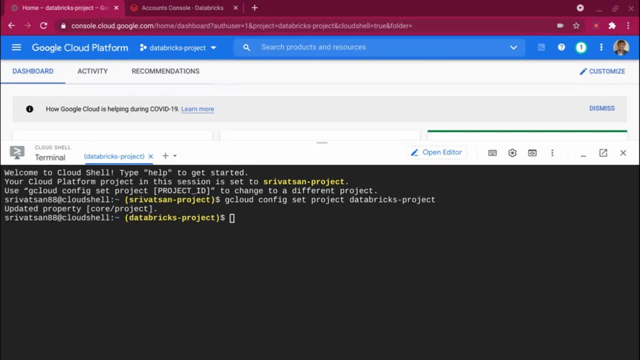 run a set of commands that will give access to all these resources. the very first thing i'm going to do is i'm going to give access to the compute nodes on google cloud platform. so, basically, this is going to enable the compute node services on google cloud platform. and after this is run, what? 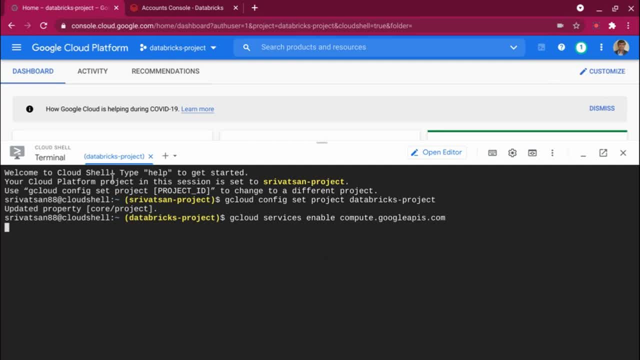 i'm going to do is i'm going to run uh- access to containers. so this is going to take some time. so what i will do is i'll open a new window and run the remaining commands over here. so i'm going to give access to containergoogleapscom so it will allow me to create containers because it's going. 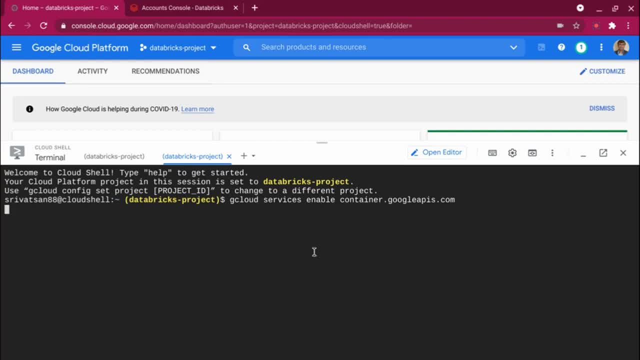 to use a kubernetes platform. i'm also going to give access to the deployment manager. so i've given access to container, i have access, given access to compute engine and now i am giving access to the deployment manager and there is one more access that is required basically, for i am services, so i'm going to run. 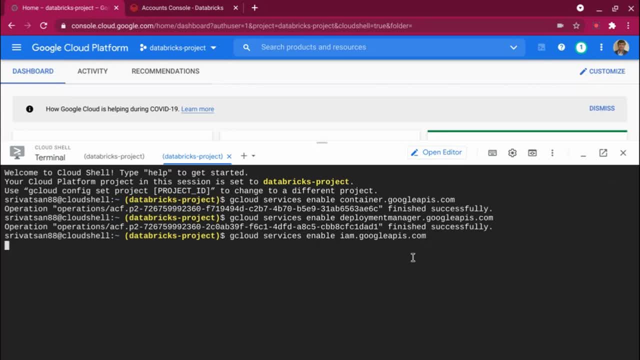 that as well. this will basically enable the i am service. so these are the four service access i need to give to this particular project so that i can create a public service over here. okay now, uh, all this, all the access, have been done. let me go to the database console and let me. 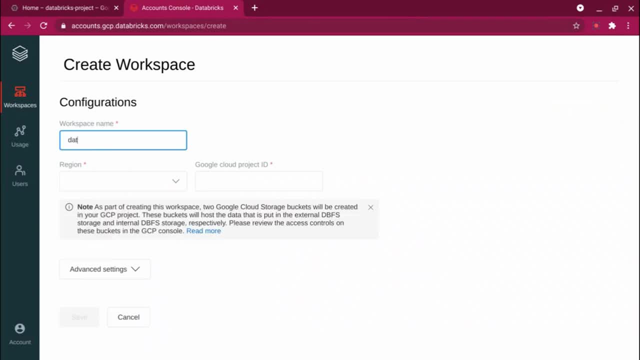 create a workspace now in the workspace. i'm just going to give a workspace name- let me give data breaks- as a workspace name, and this workspace is basically going to manage all our databricks, asserts, right? so i'm going to set a re gin that is close to me, us central one, and then i'm going to give the project name that i wanted. 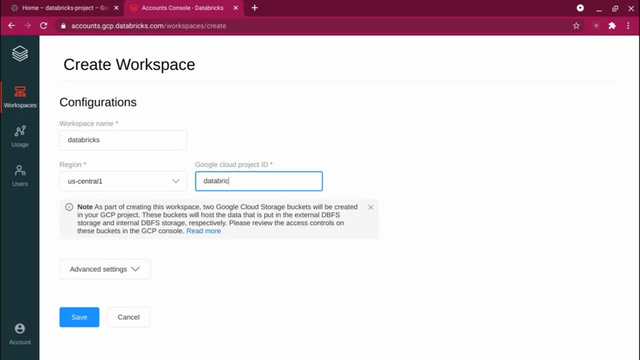 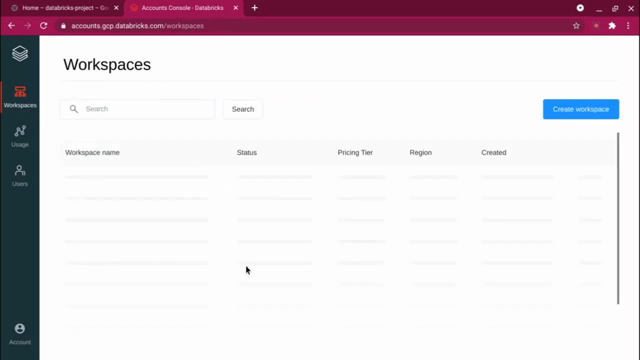 to connect to. so my google cloud project id that i created now is databricks hyphen project, so i'm going to connect to it and i'm going to say, like save. so once i click on save, it will start provisioning the workspace right now. basically, it has not created any cluster or 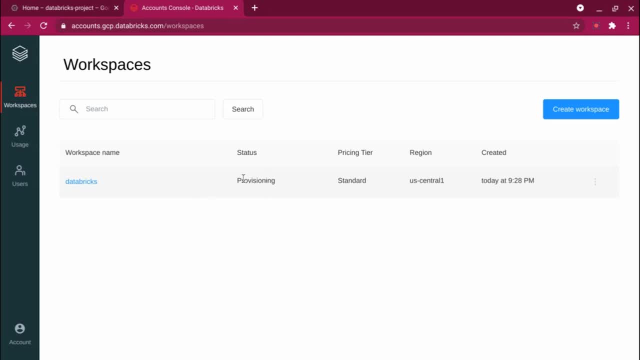 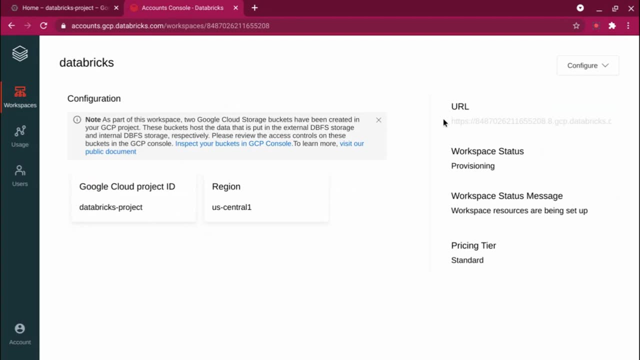 anything. it's just creating a workspace for us, so it will. this will take a few, uh, a few minutes. so once that is done, done, what i'm going to do is i'm going to go into the workspace and you can see, this url will get enabled. this url is basically the databricks, uh main console url where you can create your 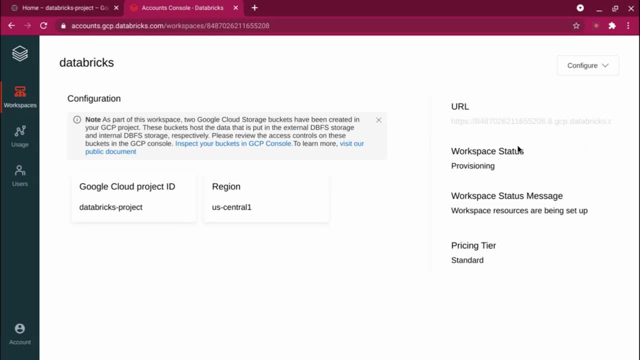 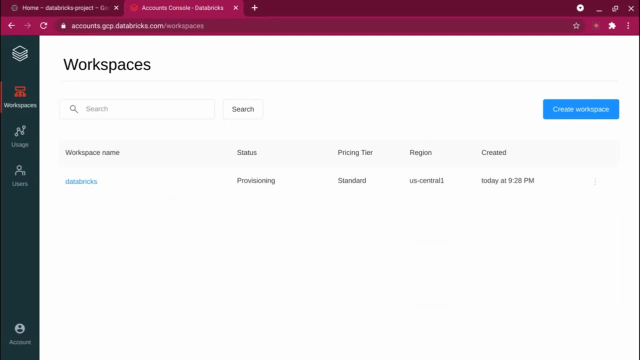 clusters where you can create notebooks, your code and everything you want to create, right? so let me go to workspace and see like uh, wow, and once it is complete i will come back to it. and now you can see, basically, the status is running and you can click on uh databricks.